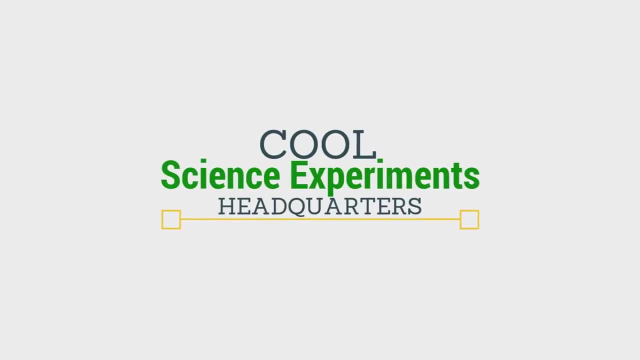 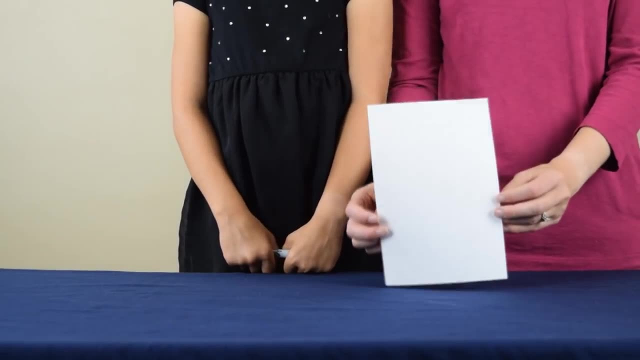 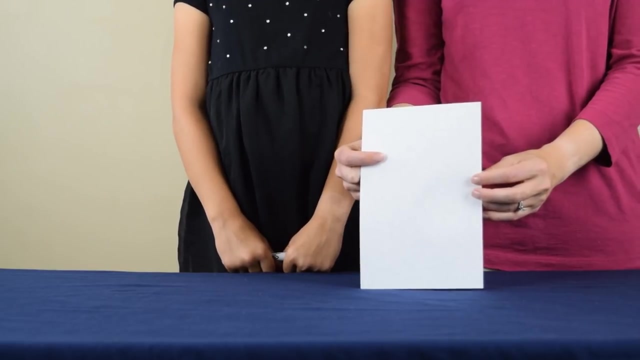 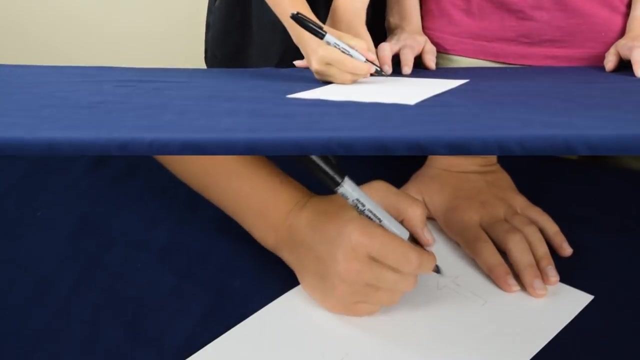 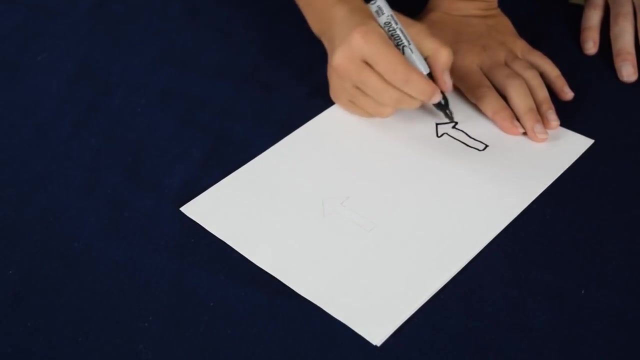 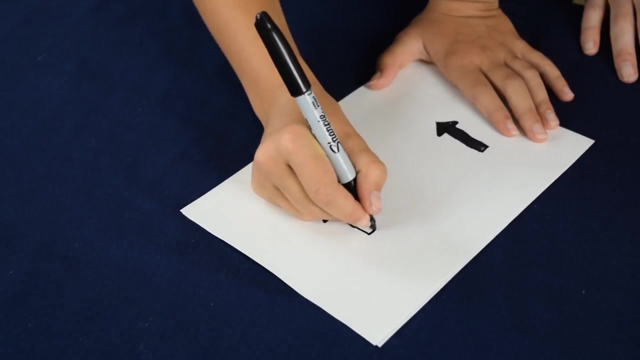 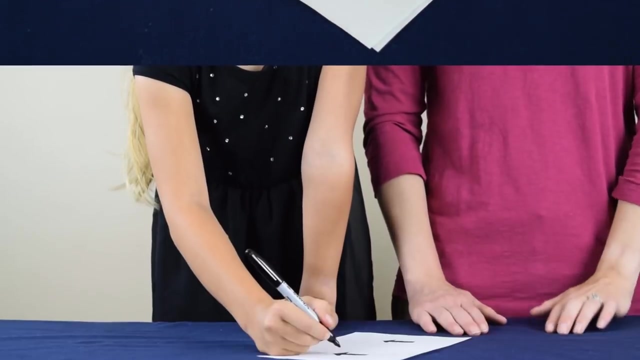 Let's get started. To begin the experiment, you're going to need a plain white sheet of paper, and you're going to draw two arrows on it: One near the bottom section and one near the top. Now that we have our arrows drawn on our paper, you can see that they're both pointing in. 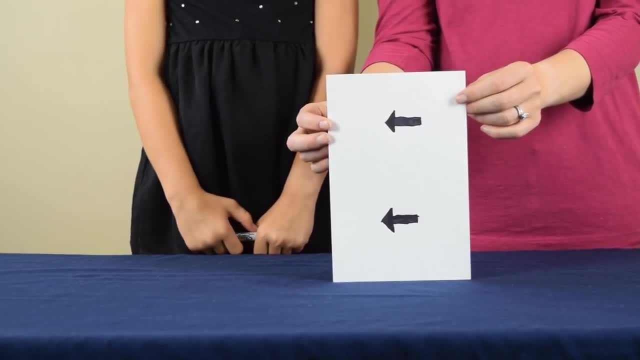 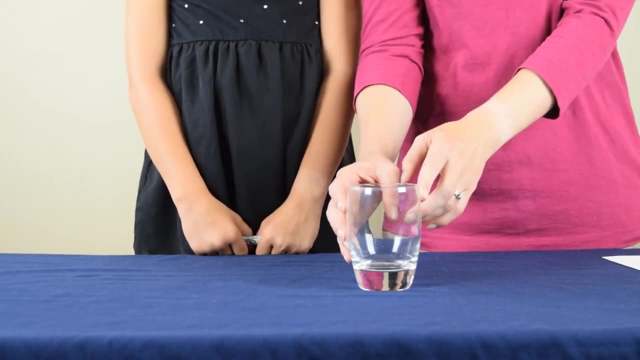 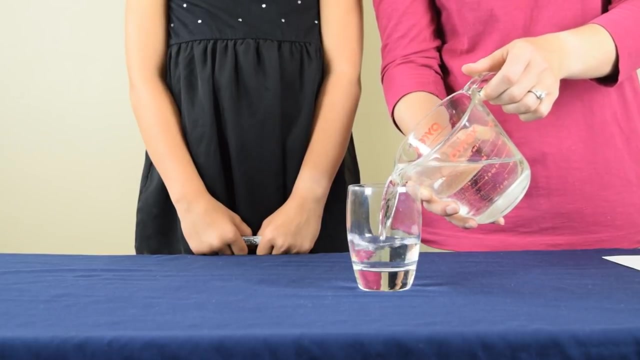 the same direction. When you have that complete, it's time to move to the next step. For this step, you need an empty glass cup And you're going to fill that cup with water. You want to make sure that you fill the cup almost to the very top. 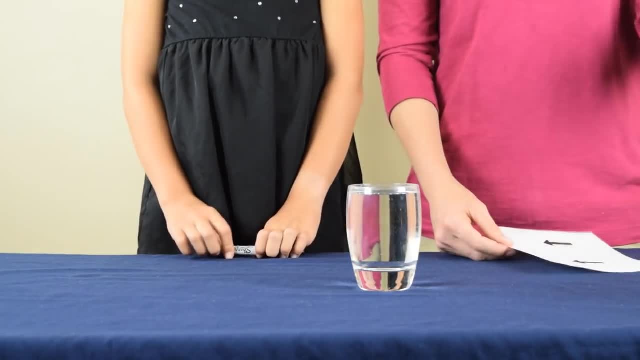 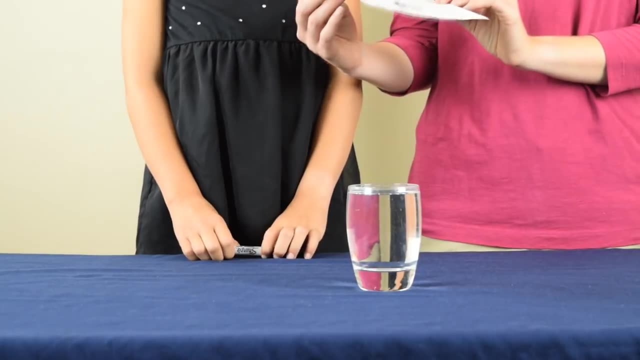 For the next step. what you're going to do is you're going to position yourself so you're looking directly into the side of the glass. Then you're going to take your piece of paper and you're going to slowly lower it behind the glass. 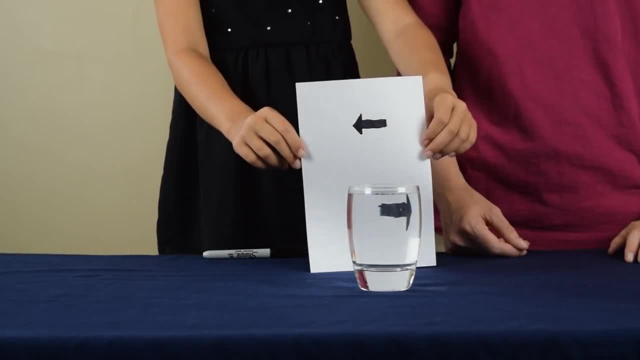 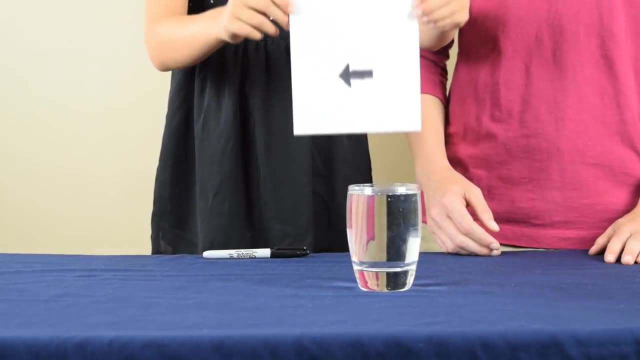 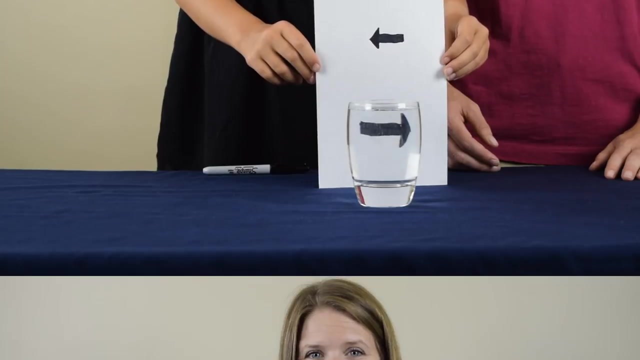 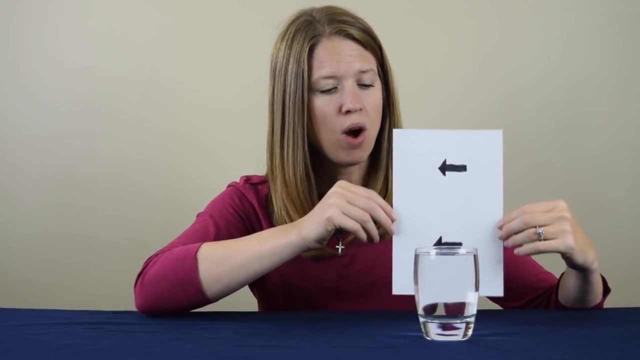 And you're going to watch to see what happens. Now let's watch that again. Raise it up and then slowly lower it down. As you can see, the arrows are both pointing in the same direction. Can you tell me why, when we look at the bottom arrow through the glass of water, does it? 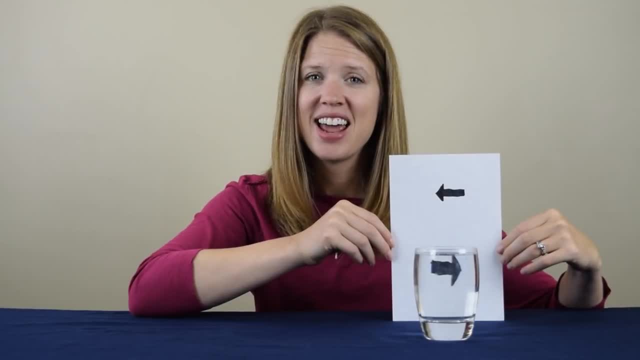 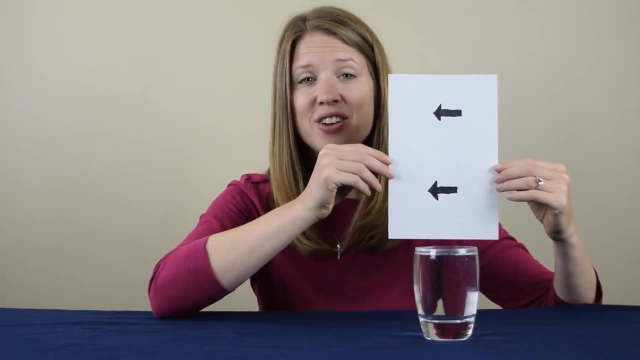 change direction. Leave a comment below to submit your guess, and then visit CoolScienceExperimentsHeadquarterscom to find out the answer. You'll be able to print out instructions for this experiment, and you can find many more that you can do at home too. 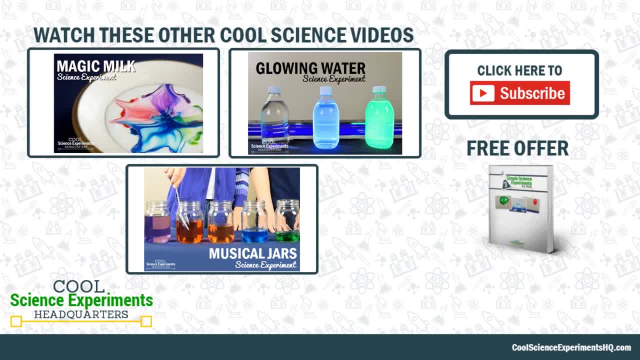